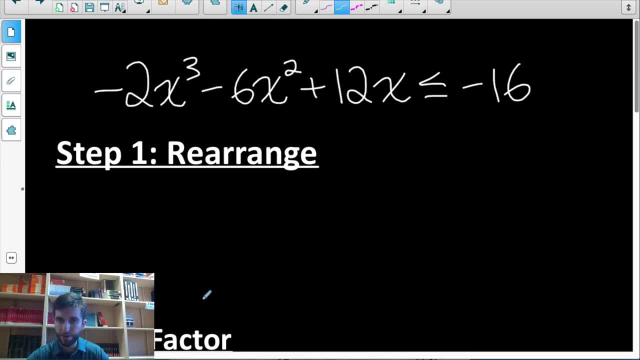 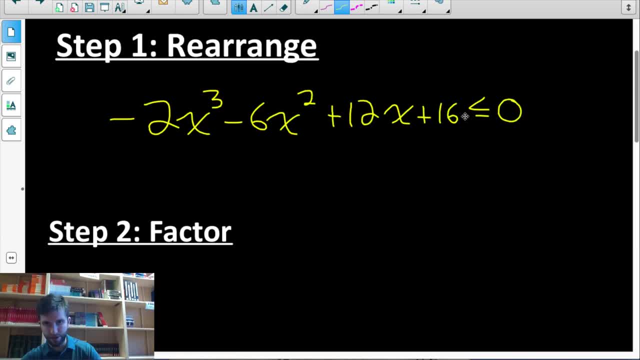 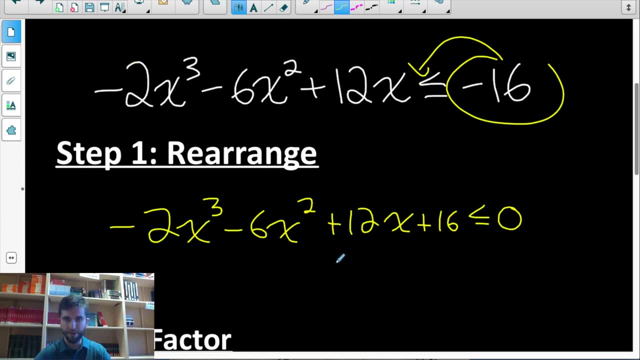 do this is because now we're interested in when is this function less than or equal to zero? and that's going to have the same set of answers as when this function was less than or equal to negative 16. but this one's a lot easier to work with because if you think about it logically now, 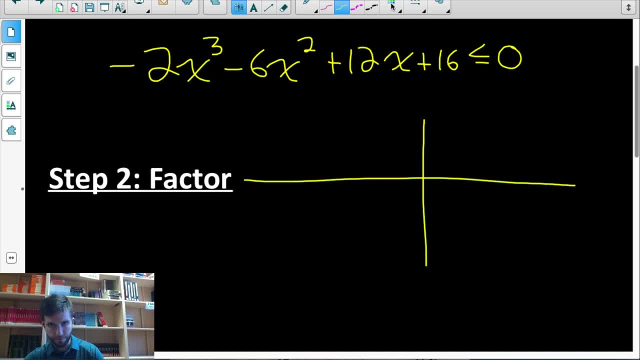 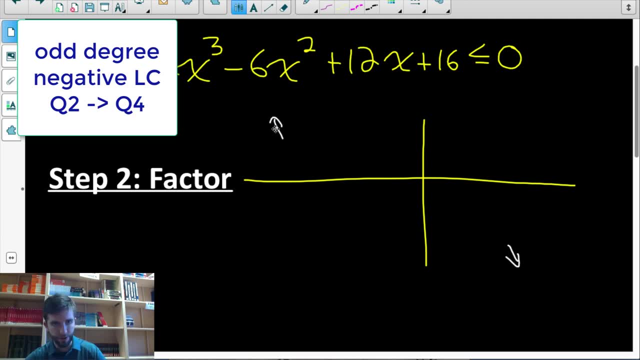 we're just interested in, well, this function. you know this function is degree three negative leading coefficient. so i know it goes from two to four and it's degree three, so it could have two turning points in between, with the y intercept of 16. so it looks something like this. we're 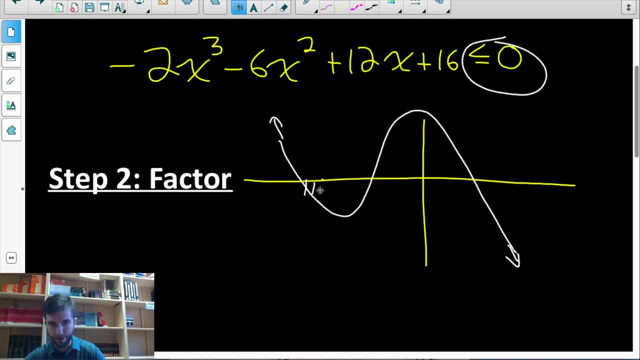 interested in when is it less than or equal to zero? so when is it below the x-axis? so i'd say in this interval and this interval. now this graph isn't perfectly accurate, but you can see why having it set less than or equal to zero is useful, because then we're just looking for when are the 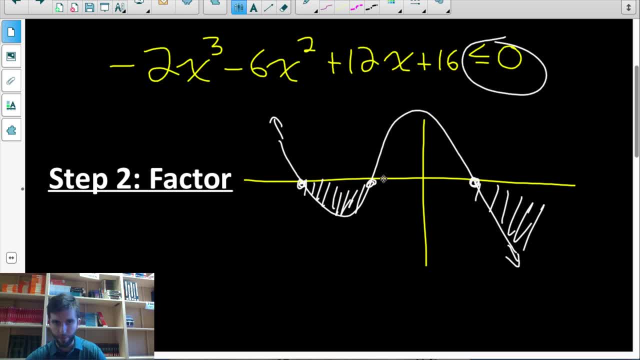 y values of the function less than or equal to zero? for what range of x values is this true? so, in order to be able to graph this perfectly accurately, accurately, we're going to have to find what are these x intercepts here, where the function switches from being positive to 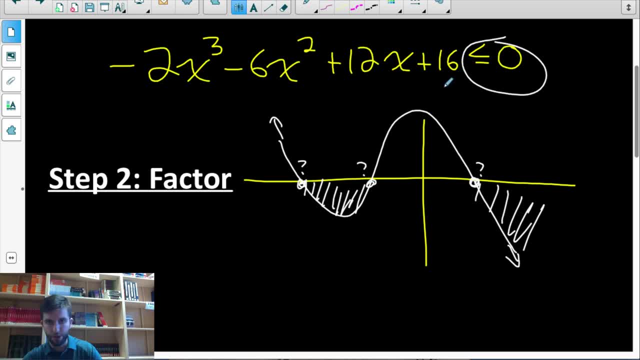 negative or vice versa. so if we want to find the x intercepts, you know by now that we need to get this into factored form. so that's why step two is factoring the polynomial. so in factoring, step one should be always to check for a common factor. so i noticed that i could common factor out negative. 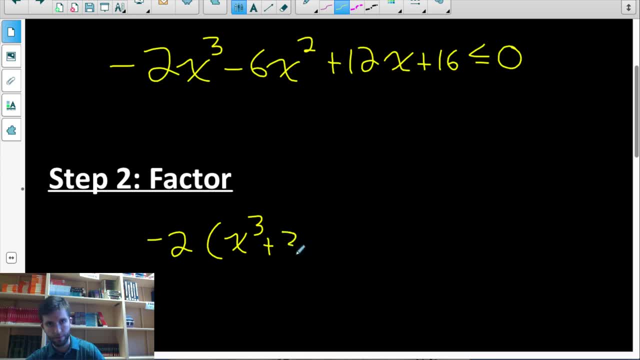 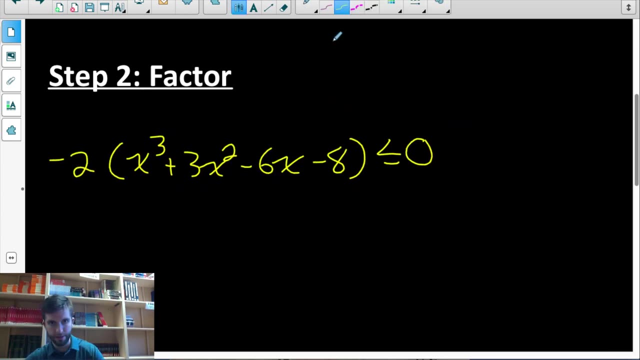 two from all of the terms: x cubed plus three, x squared minus six, x minus eight, less than or equal to zero. and now i'm interested in factoring what i have inside here further. i want to get into fully factored form so i can find the. 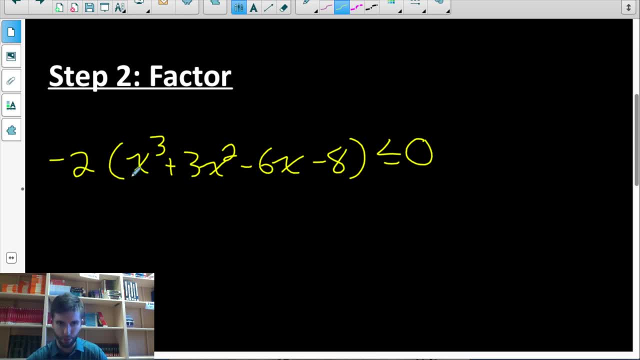 x intercepts, so it's four terms. so i would try grouping. but you'll notice grouping won't work with this. we wouldn't get a common binomial. so when that happens you're going to have to test for zeros into your synthetic or long division to get it into factored form. so i'm going to want to 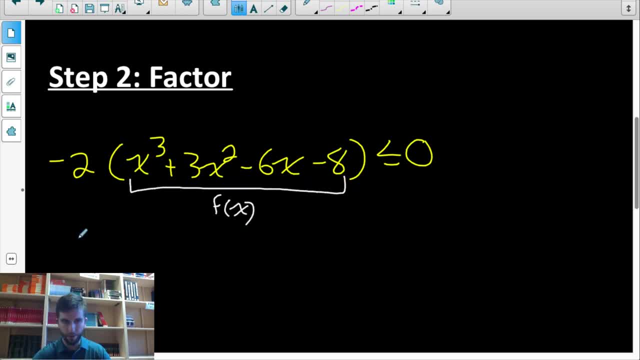 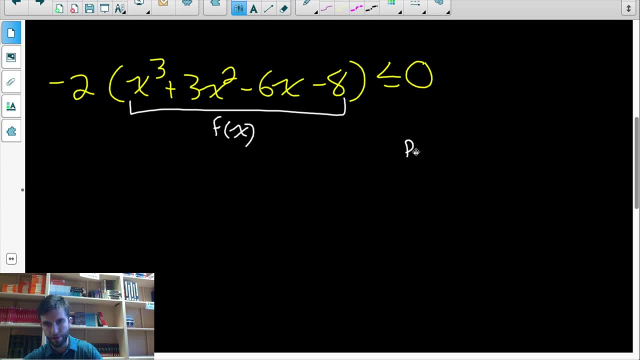 try and factor this further. i'm just going to call this f at x to keep my work organized. now we need to try and guess and check integers that could make this into factored form, so i'm going to call this zero. and the only integers that could work- so i call these possible zeros- are factors. 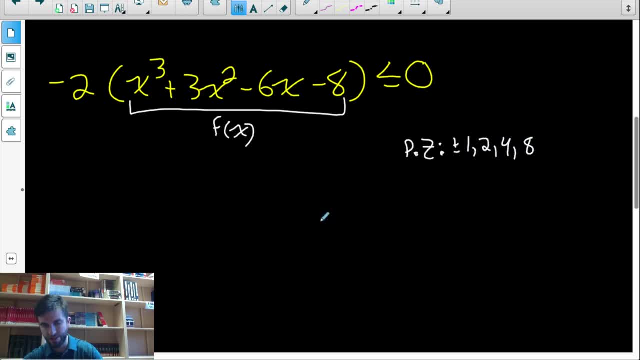 of eight. so plus or minus one, two, four or eight, those are the set of integers that could make this become zero. we just have to test until we find one that works. if we plugged one in for x, you know it wouldn't equal zero. but if we plug negative one in for x, i would get negative one plus three plus. 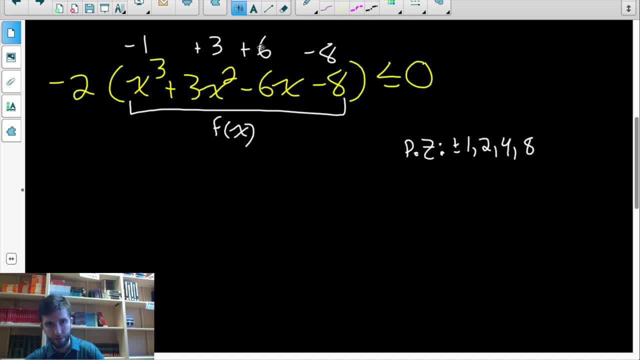 six minus eight. so that's two plus six is equal to zero. so if we plug negative one in for x, that's eight minus eight is zero. so i just figured out that f at negative one equals zero. so that tells me that x plus one is a factor of f at x. so i can off to the side here. i can divide this polynomial. 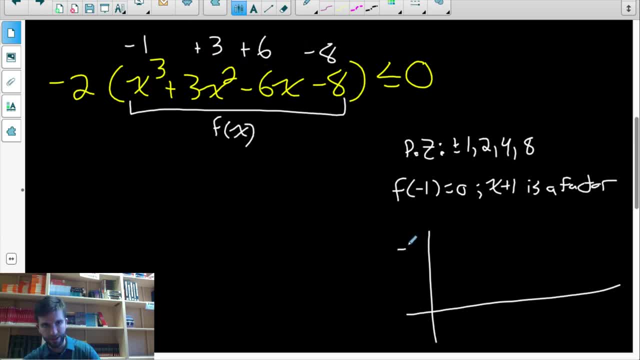 here by x plus one and i'll use synthetic division. i think that's a little bit quicker. so i figured negative one was the zero. the coefficients of the function are one, three negative, six negative, eight. do the synthetic division quickly: negative one times. one is negative. one, three plus negative. 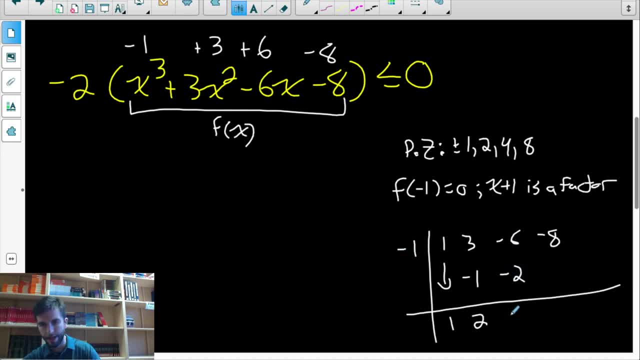 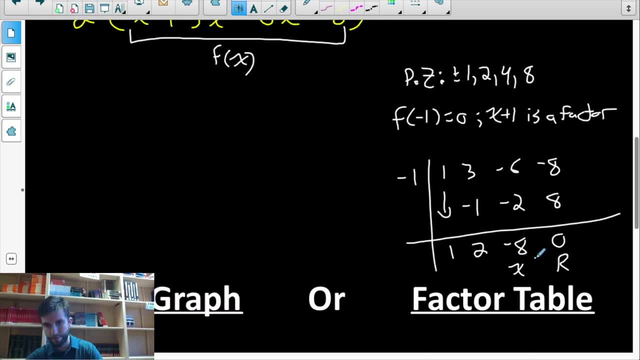 one is two, and i'm going to divide this by x plus one, and i'm going to divide this by x plus one. two negative one times two is negative. two add, get negative, eight, multiply, get eight, and there's my remainder of zero. so what i have here is my remainder, my x to the zero term, my x to the one. 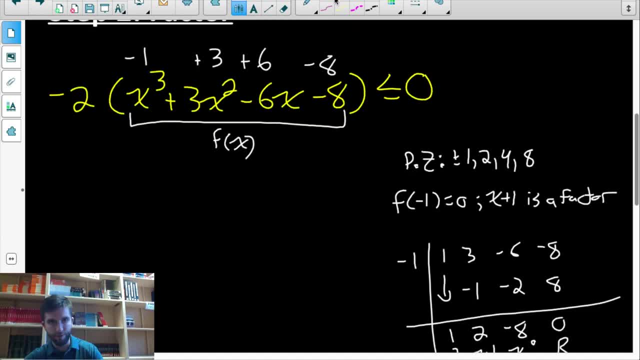 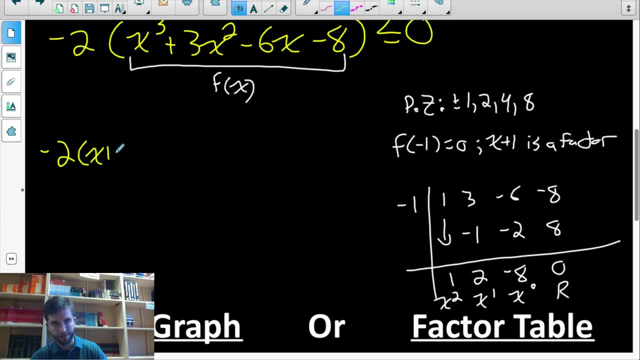 term and my x to the two term that are in my quotient. so i can now factor this to negative: two x plus one times my quotient. x squared plus two x minus eight, with no remainder of zero. so i can now factor this to negative two x plus one. 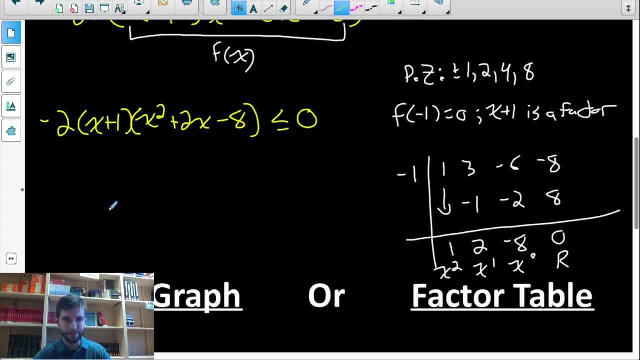 less than or equal to zero. now that it's in factored form, oh, i can factor this one further. right, this is a degree two polynomial, so it's a quadratic. i can factor that further if i can find numbers that multiply to negative eight and add to two. and those numbers do exist. they are: 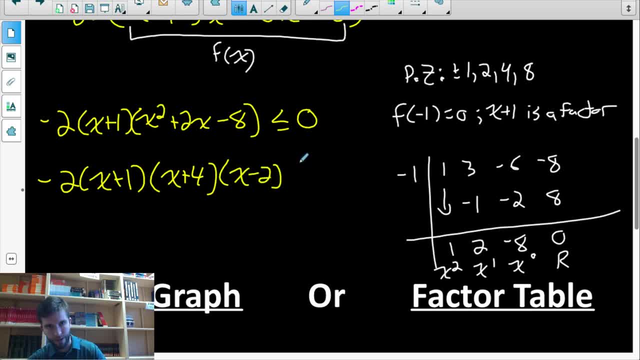 four and negative two. so there we go. now that's fully factored form right. each factor is degree one and i have this constant factor in front. i could divide that over, but then i'd have to reverse the inequality. so i'm just going to leave it there and i'm going to divide this by x plus one. 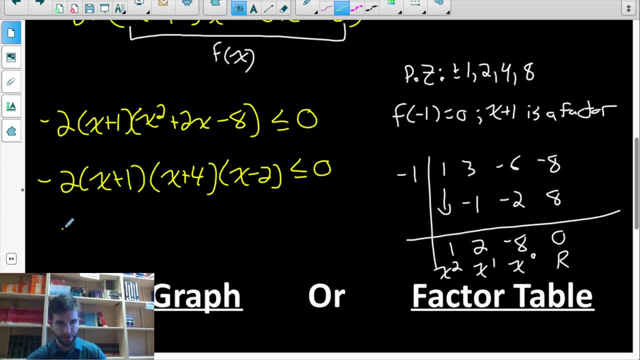 and i'm going to do that just to keep this as straightforward as possible. so i know this function has x intercepts at x equals negative, one negative, four and two right. each of those values would make, each of those values would make this whole product become zero. so this tells me. 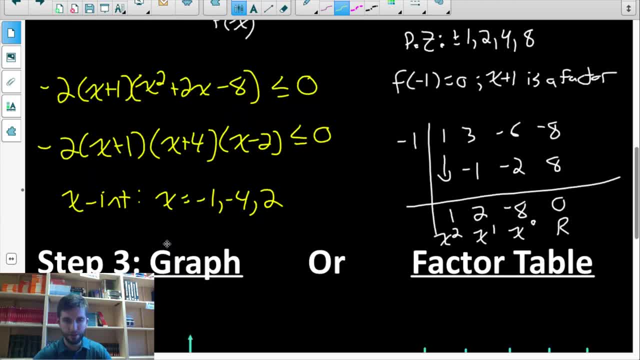 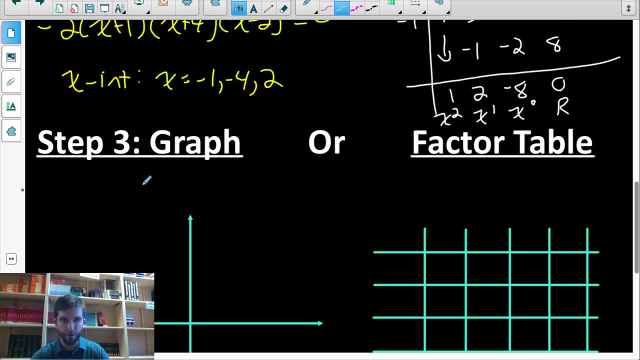 when it's equal to zero. but i want to know when is it less than or equal to zero? so we're going to use those x intercepts as the dividing points, either in our graph or in a factor table. so i'll show you both methods. so our graph: we know there's x. 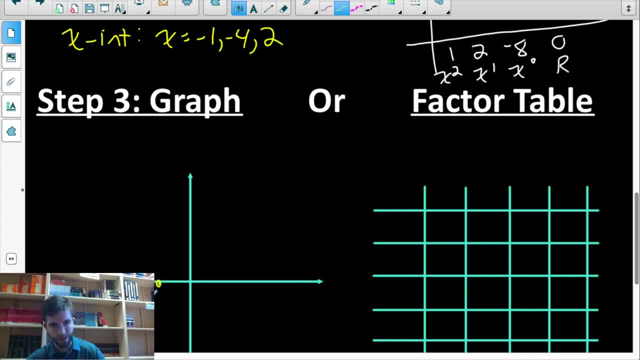 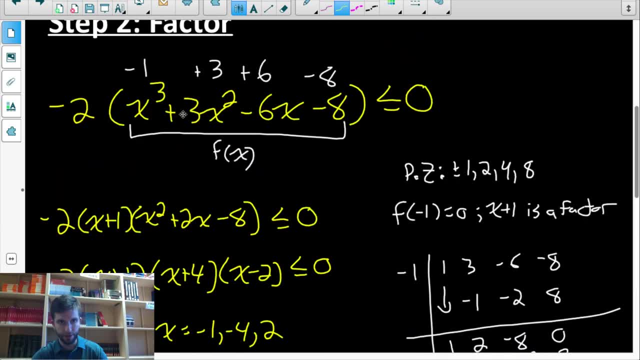 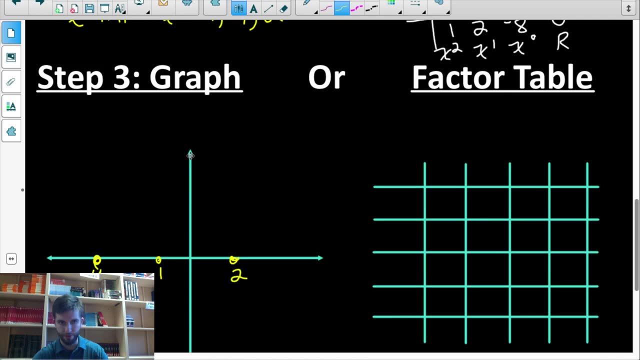 intercepts. i'll just roughly plot them at negative four, negative one and two, and the function. remember, this is the factored form version of, so it's the factored form version of this function. so it had a y intercept of 16. so let me just roughly plot that as well. i mean the y intercept isn't really useful. 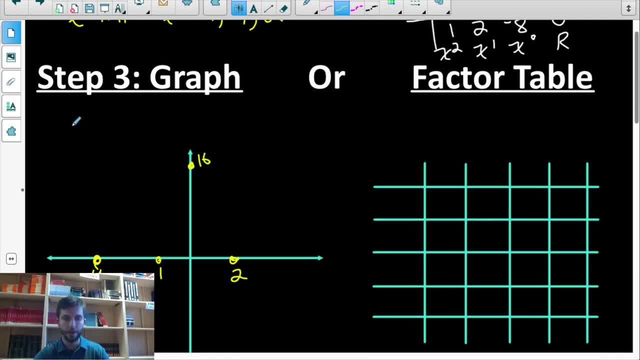 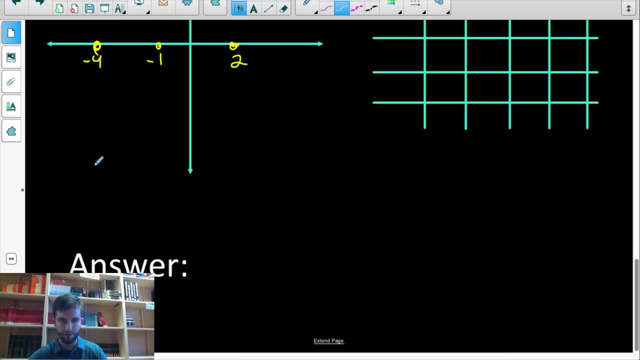 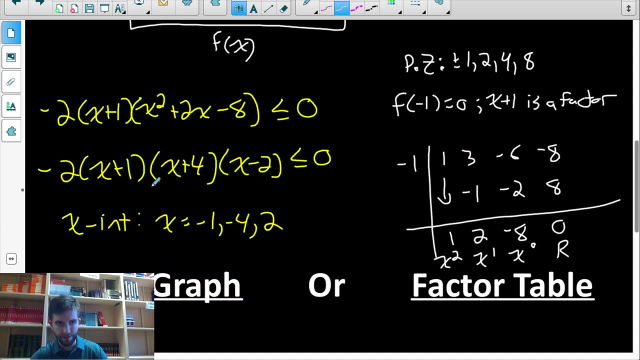 for this, but just to keep the graph as accurate as possible and remember that function up there- we already talked about it. it was a negative leading coefficient and an odd degree. so we know that goes from q2 to q4. so i know it's going to go from here to here and if you look at each of the factors, each of the 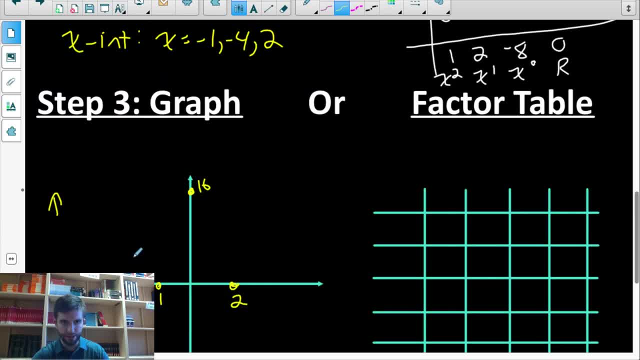 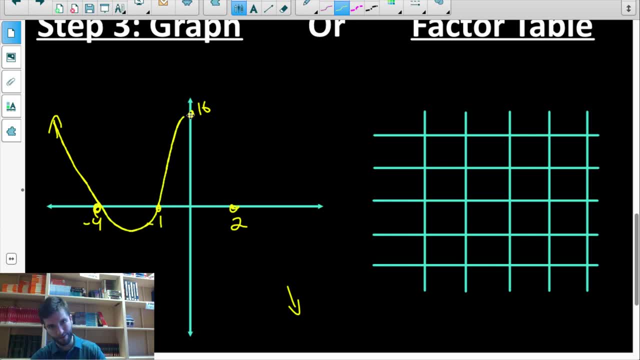 factors was order one, so i know it's going to go straight through at each of the x intercepts. so the function is going to look something like this. so that's a very rough sketch of what the function would look like. and now we're interested in 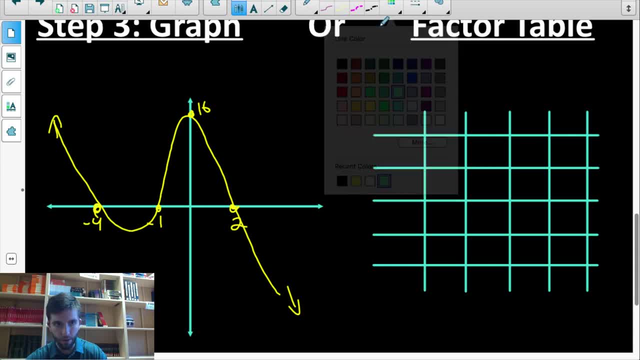 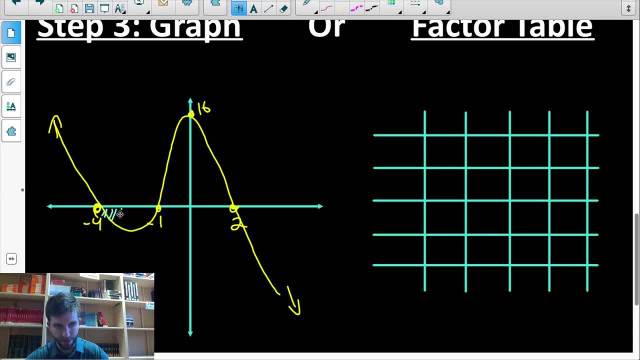 explaining when is this function less than or equal to zero? so for what x values do the y values of the function go to zero or below? so we would be interested in this part of the function and also this part of the function in those two intervals between x values of negative four, negative one, and between 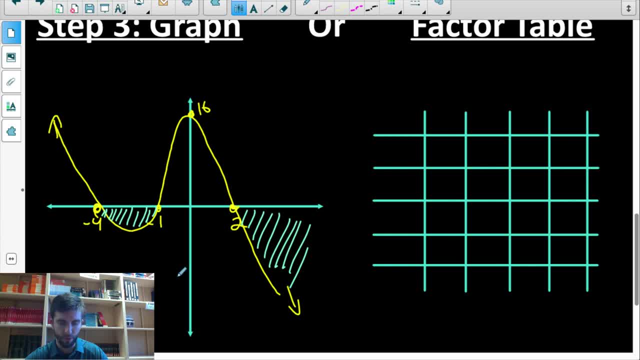 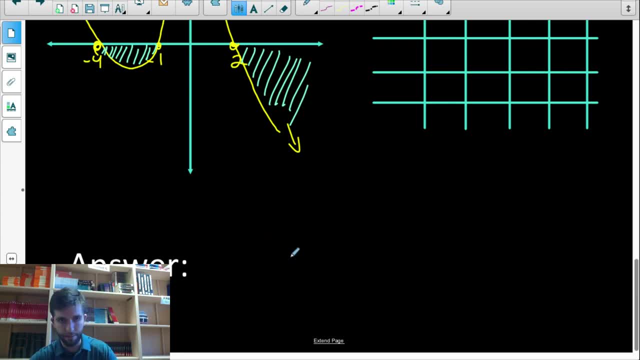 two and infinity, the y values of the function would be negative. so that's going to be the answer to our inequality. so now we can write our answer in two different ways. we could write it in bracket notation, so it's between negative four and negative one. so we want to describe our interval. 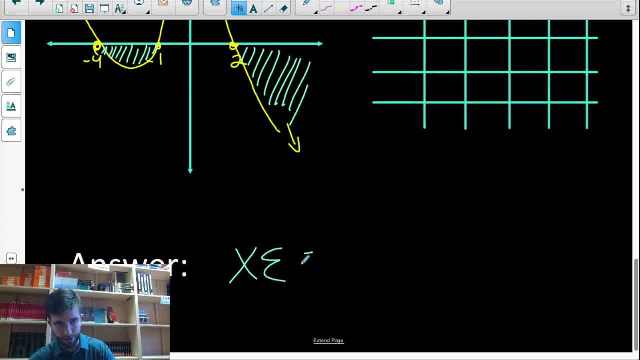 as true when we have an x value, that is an element of numbers, between negative four and negative one, including negative four and negative one. that's why i have the square brackets. or if we have an x value between two and infinity, including two, round bracket at infinity, always a round bracket at. 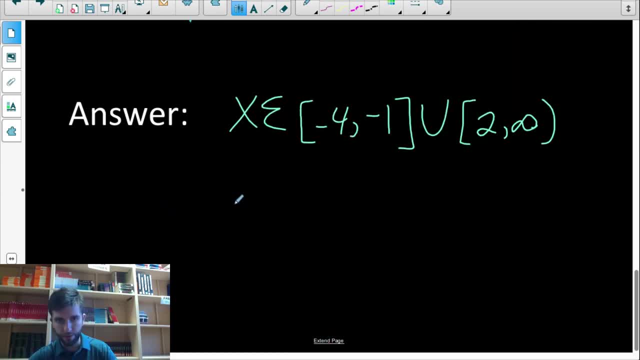 infinity, or we could write this as an inequality, we could say, between negative four and negative one, including those two. that's why there's the equal sign under. x is greater than or equal to 2.. So hopefully you understand why this is the answer right. 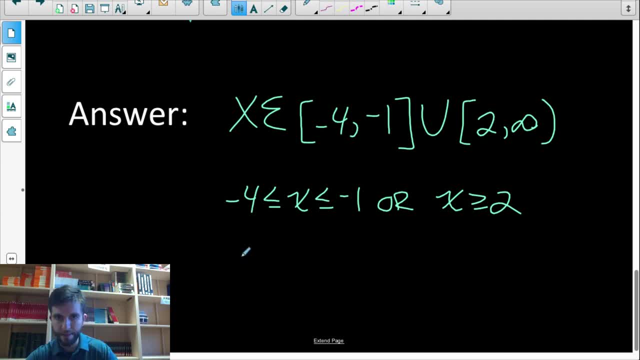 These are the x values that make the original inequality true. These are the input values. so if I input a value into the original inequality that is within this interval or this interval, it'll make the inequality true. So let me give you a better graphical representation. So this: 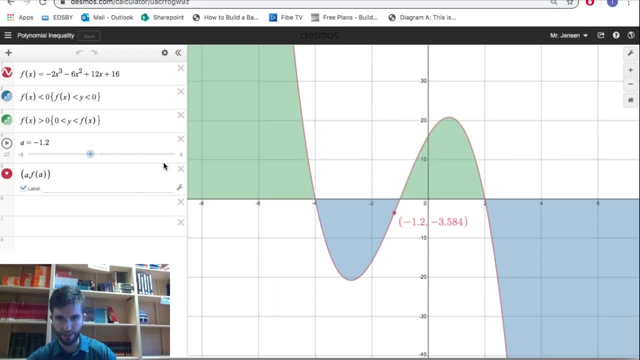 is just a very rough graph. Let me show you what the Desmos graph looks like. So here's the same function graphed on Desmos and you'll notice while I'm moving the slider here. just take a look at the point. So the point has the x value and the y value. So look between negative 4 and. 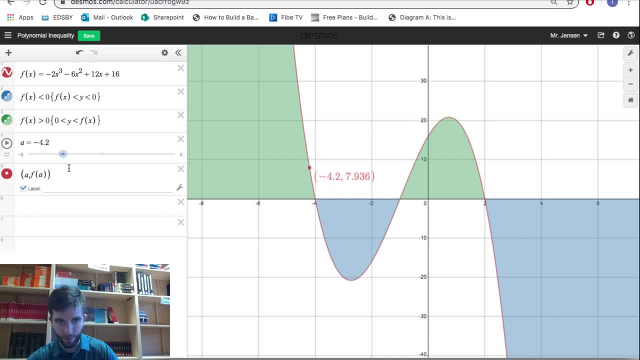 negative 1, and I'm talking about x values- between negative 4 and negative 1.. Look at what the y values are. The y values are all negative. The y values are all negative between negative 4 and negative 1.. But what about when we go to x values- between negative 1 and 2?? Well, the y values are: 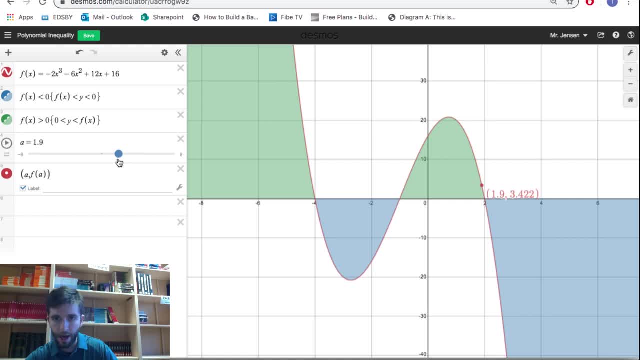 all positive there, right, The function's above the x-axis. And then what about for x values bigger than 2?? Well, all the y values are all positive. So what about when we go to x values? between y values are now negative. so the original question wants to know when is? 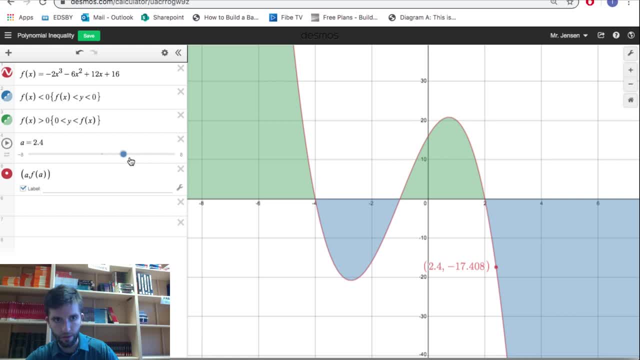 this function less than or equal to zero. so when are the y values negative? for what x values? are the y values negative for x values between negative 4 and 1, and also for x values bigger than 2, and now notice we included negative 4. 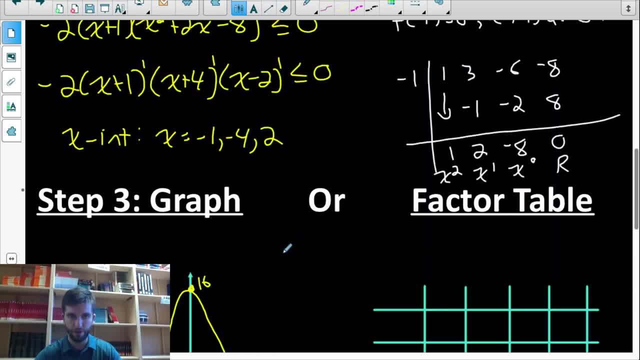 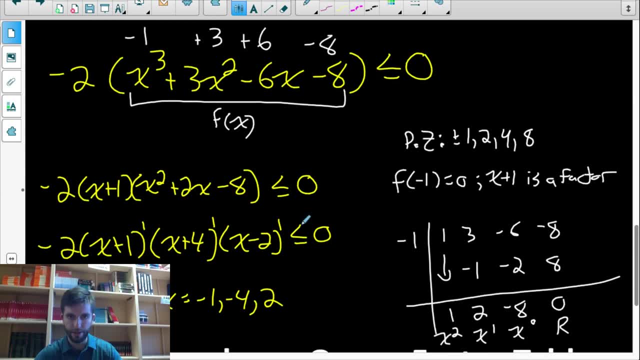 negative 1 and 2 in our answer because the funk. the original question wants to know not only when is it less than 0, it also wants to include the times when it's equal to 0. so in our final answer, that's why we put square brackets in our 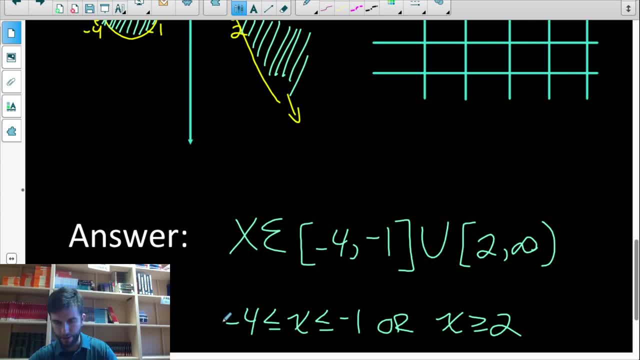 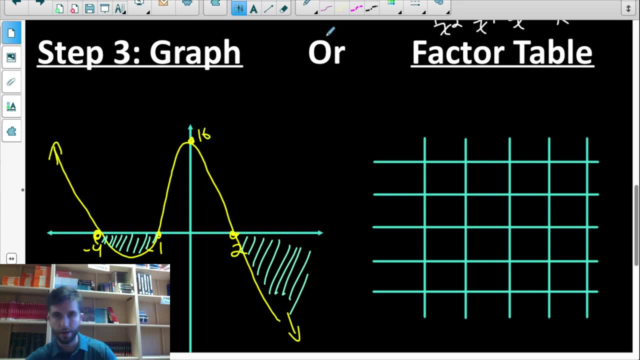 bracket notation, or when we wrote it as inequalities, we put lines underneath. so now let me show you how we could get the exact same answer using another method called a factor table or sign chart. and how does that work? well, at the top of it we put negative infinity on the left, we put infinity on the far right and 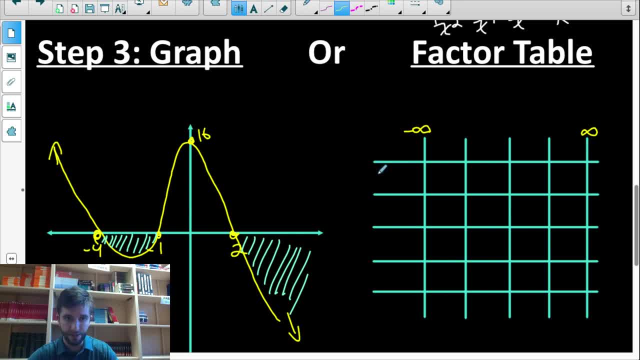 between it. what we do is we divide it up into intervals based on where the X intercepts are. well, we figured out the X intercept. we're at negative 4, negative 1 and 2. so negative 4, negative 1 and 2, and basically, 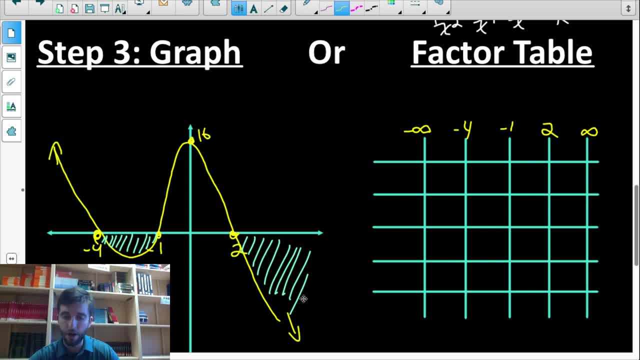 what we're going to do. instead of actually graphing it and looking at the graph, we're just going to choose test points and plug those test points into the original equation and figure out are the Y values positive or negative, without actually having to look at the graph. so we're going to have to choose a test. 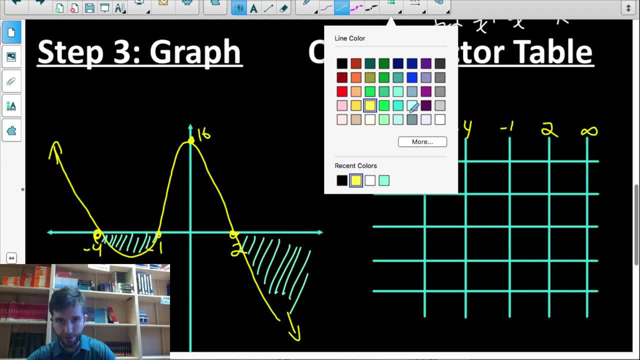 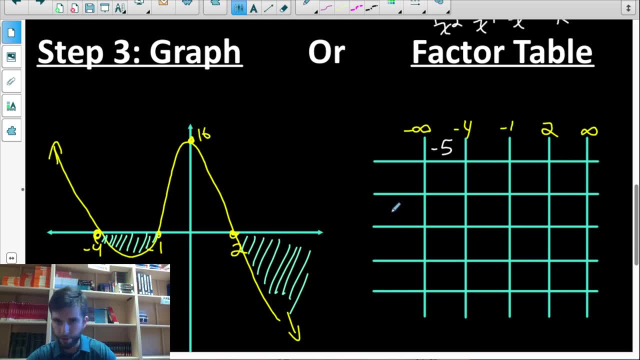 point within each interval. so I'm going to choose some test points in each of these intervals now. so between negative infinity and negative 4, I'll choose negative 5, but you know negative 10 would have worked as well, and between negative 4 and negative 1, I'm. 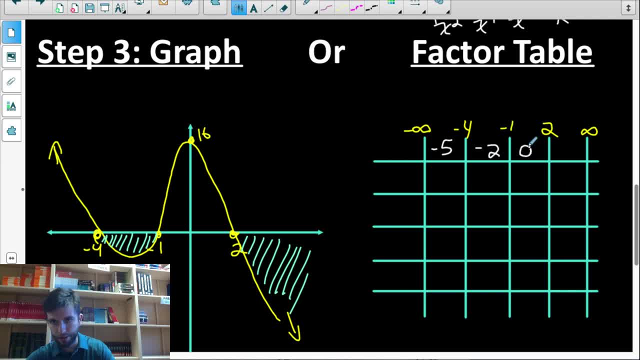 going to choose negative 2. between negative 1 and 2, I'm going to choose 0, and between 2 and infinity, I'm going to choose 3. so these are all X values that we are going to input into the function and test whether the function is. 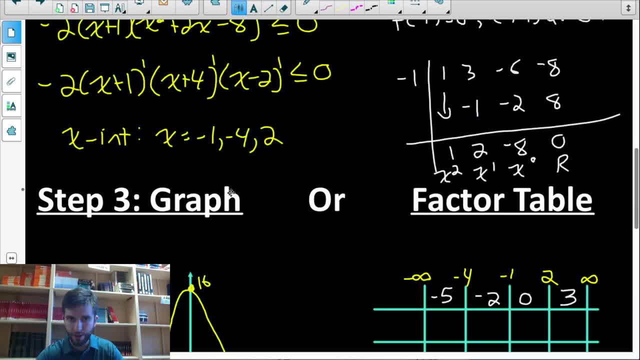 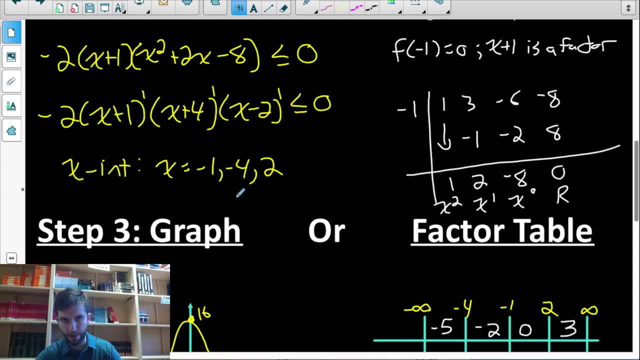 positive or negative. and when we test it in the function, we're going to do it in a bit of an organized way. we're going to test it in each of the factors separately instead of plugging it into the entire original function and then evaluating it. it's actually easier if we plug it into each factor separately. 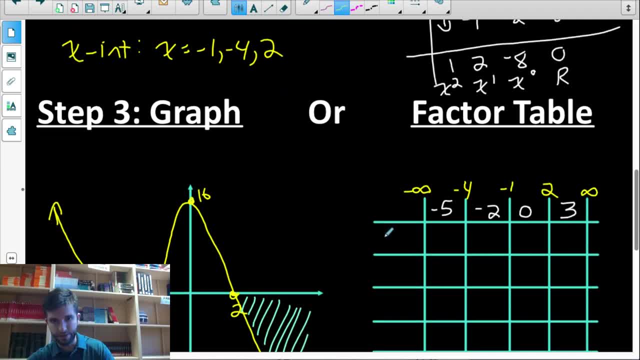 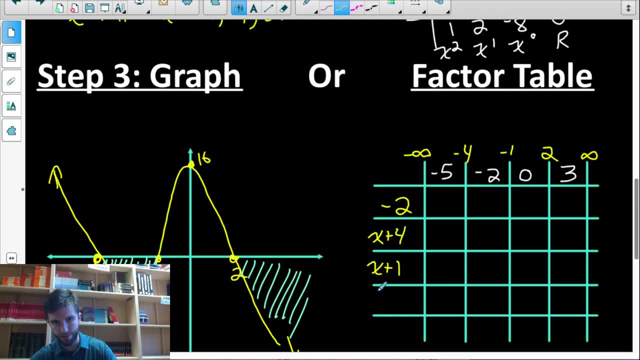 let me show you what I mean by that. so we put each of the factors down the side here. so negative 2 was a factor of our function, X plus 4 was a factor, X plus 1 was a factor and X minus 2 is a factor. and now what we do is we test each of. 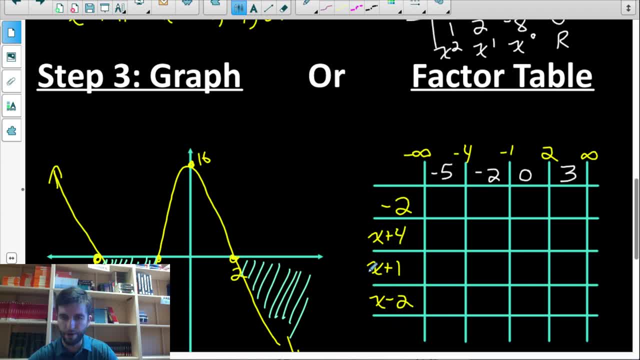 these numbers into each of these factors and then just record whether our result would be positive or negative. so well, negative 2 is always negative. I could just complete that real quickly. so when negative 5 is plugged into X plus 4, I would get negative 3 and negative 5 equals positive 4, because we're going to 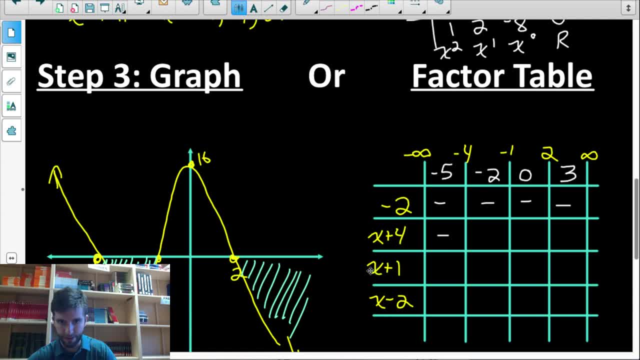 get negative 5 plus 4,, which is negative 1. When negative 5 is plugged into x plus 1,, I would get negative 5 plus 1,, which is negative 4. And negative 5 minus 2 is negative 7. So notice what we have. 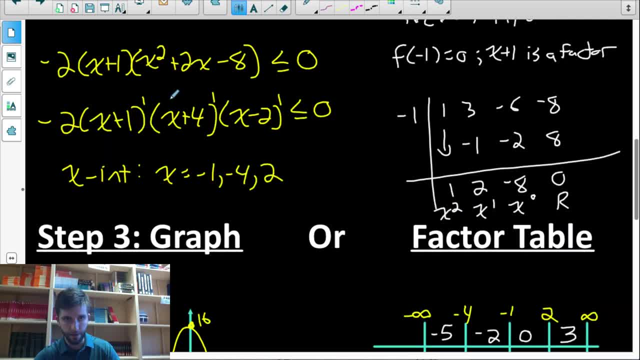 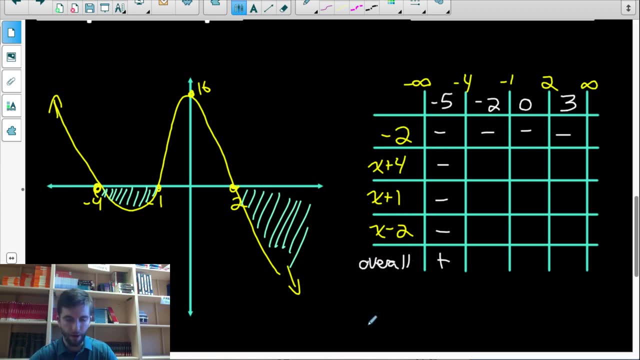 figured out here is that each of the factors in this factored form equation here would become negative. So I would have a negative factor times a negative factor, times a negative factor times a negative factor. An even amount of negative factors gives us an overall result of a positive function. 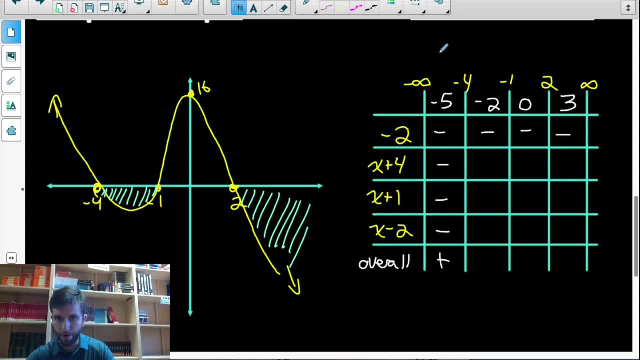 Meaning that it is bigger than 0 at that point. So this is not part of our answer. Notice the function in that interval we just tested in the negative infinity to negative 4, the function is positive. This part of the function all has positive y values. Well, how about between negative? 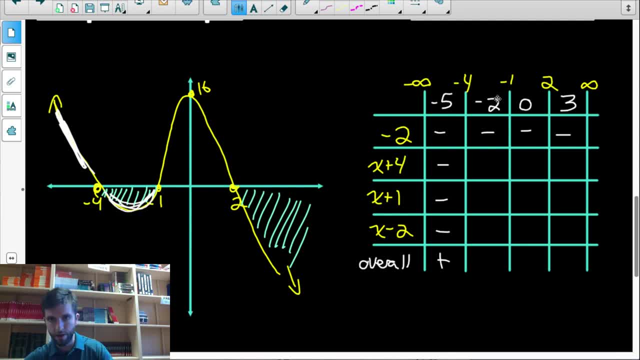 4 and negative 1? How about this part? What are all these y values? So we test negative 2 into the function And it makes this factor positive, It makes this factor negative. It makes this factor negative. An odd number of negative factors results. 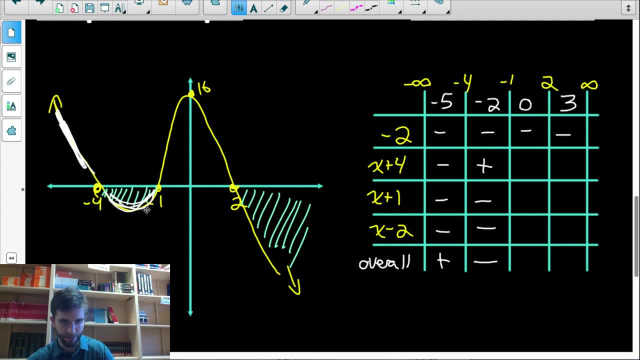 in a positive function. So we have a positive function And we have a negative function, An overall function that is negative. And notice, yes, all the y values are negative there. How about 0?? Positive, positive, negative. We have two negative factors, which results in a positive. 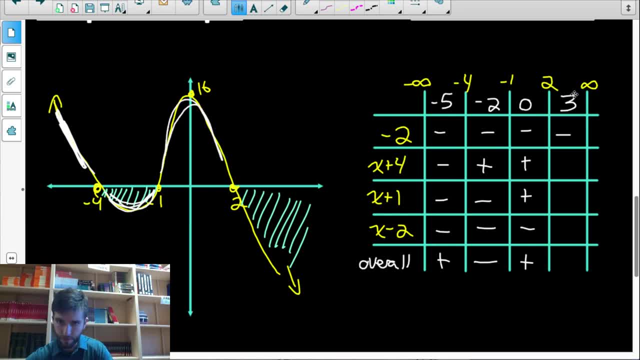 function And look, the y values in that section are all positive. Test 3,: positive, positive, positive. So we have one negative factor which means the original function has negative y values in that section. So we just use the x-intercepts as the dividing points And then choose test. 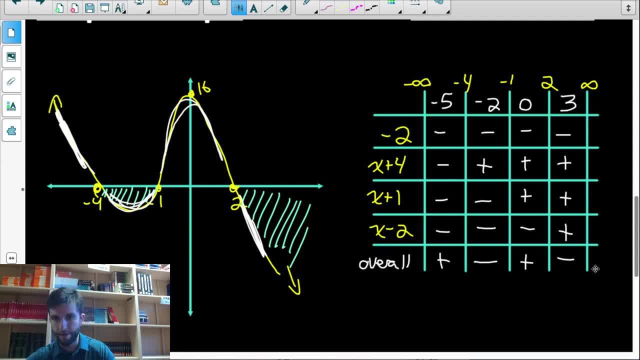 values in each interval, Plug them into the function And we have a negative function. We want to find the factors of the original function And figure out the sign of the original function And notice how this table reveals the final answer to us, The original question.